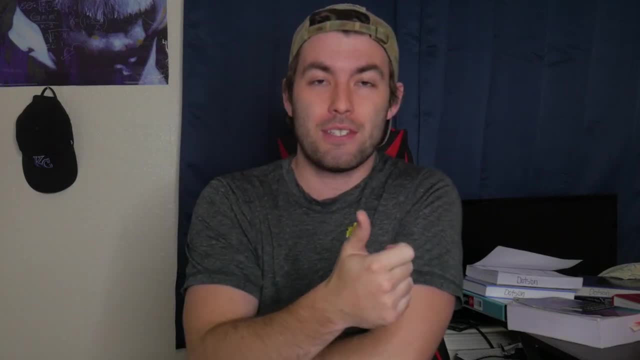 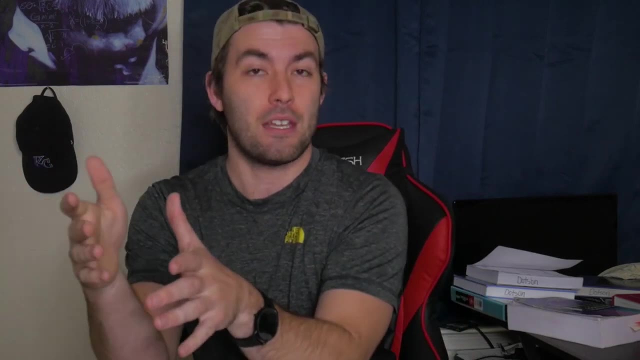 Well, think about it. In undergrad you have to have your introductory physics course, which is just one big old course on classical mechanics. It's one big course on Newton's laws. Then you have to take an advanced classical mechanics course in undergrad, Then in grad, 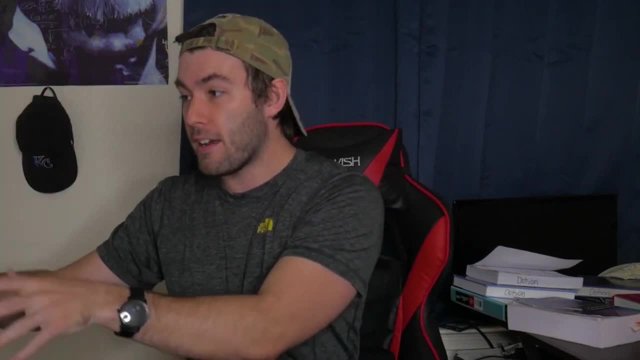 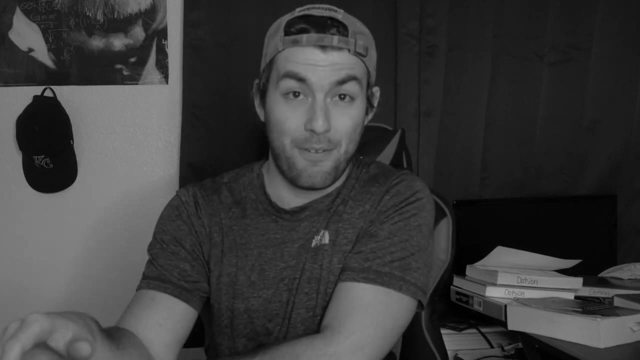 school, you have to take classical mechanics again even deeper, And then and then nothing. This is the last classical mechanics homework I will ever have to do for the rest of my life. So for the final time, let's talk about what this week's classical mechanics homework will be on. 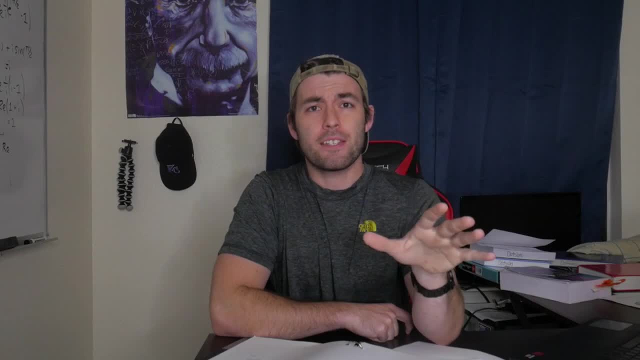 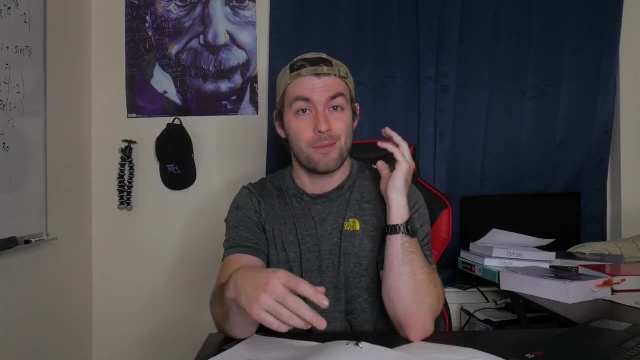 Don't cry. Don't cry, It's a happy time. This week's classical mechanics is all on the Hamiltonian formalism And a lot of your classical mechanics. you'll spend it with the Lagrangian approach, where you have some generalized, coordinate, generalized. 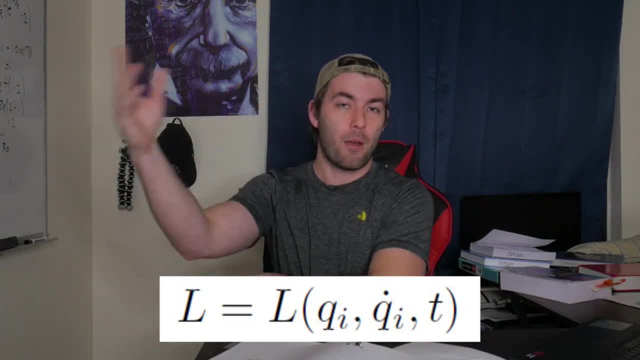 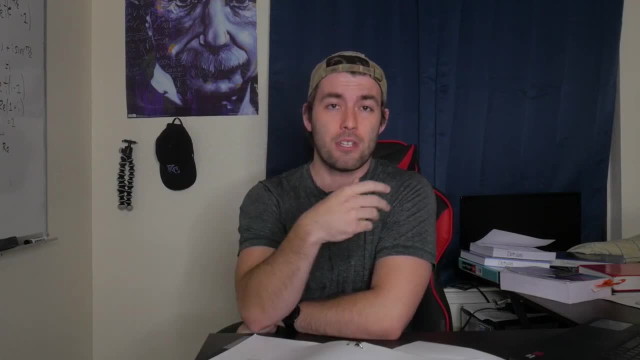 velocity. You solve the Euler-Lagrange equations of a system and come up with the equations of motion. You can do the same thing for Hamiltonian formalism. They're very similar. They have their differences. For one, instead of generalized coordinate and velocity, the Hamiltonian is. 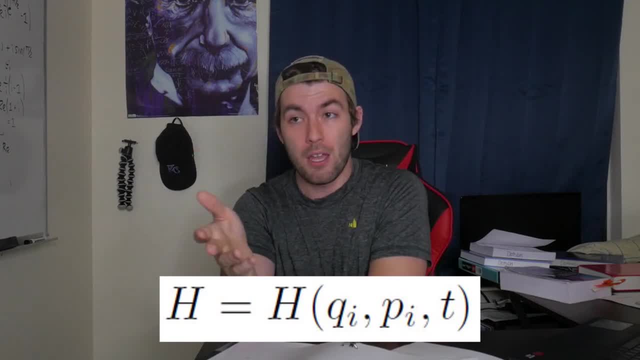 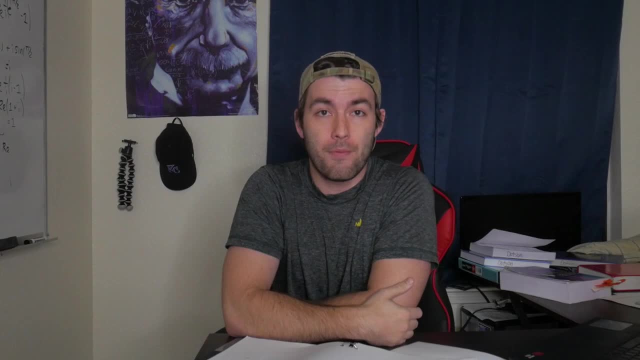 represented by some generalized coordinate and some generalized momentum. You might think: what's the difference? Can't I just multiply the velocity by some mass? Not exactly. For example, in electromagnetic theory you can have some momentum of a charged particle. that has to do. 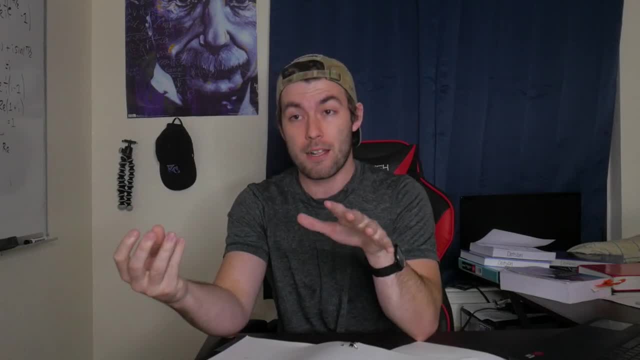 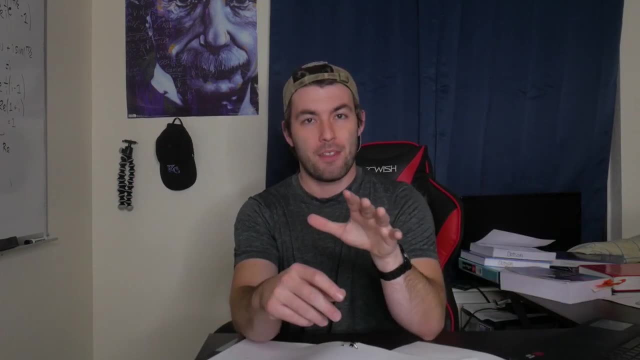 with its mass and its velocity. But there's also a contribution, the fact that the electromagnetic field exists. The electric field is contributing to the momentum itself. So in general you can't just multiply by the mass and think that that's the momentum. 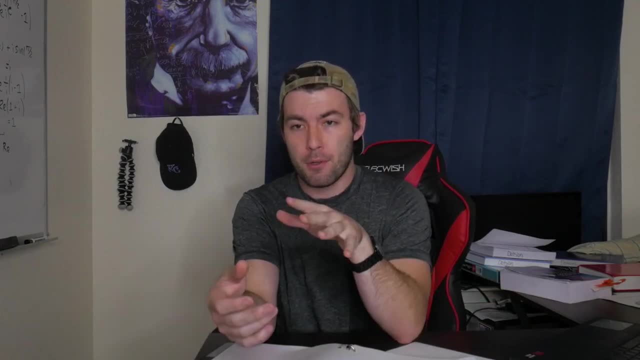 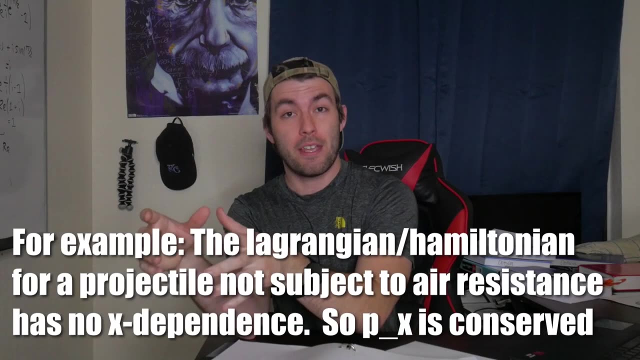 The Hamiltonian and the Lagrangian all have their benefits. For example, for the Hamiltonian, which is a function of generalized coordinates and generalized momentum, if you have a cyclic coordinate which means it doesn't show up in the Hamiltonian, well then that also means that the 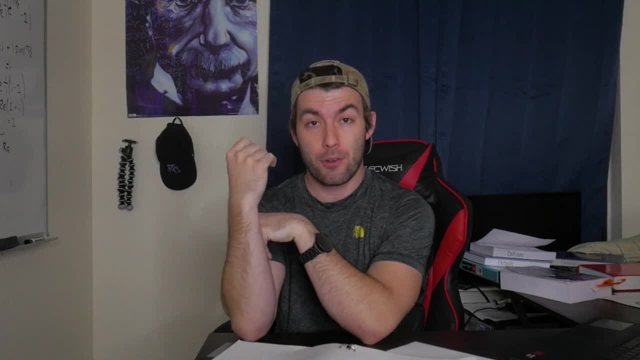 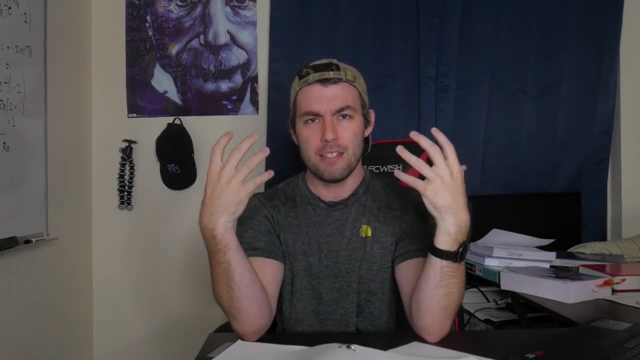 generalized momentum is conserved. So if you have something that's a function of your generalized coordinates and momentum and you just found out that one doesn't show up and one is just a constant, then that makes your life a whole lot easier And that really isn't as helpful in the 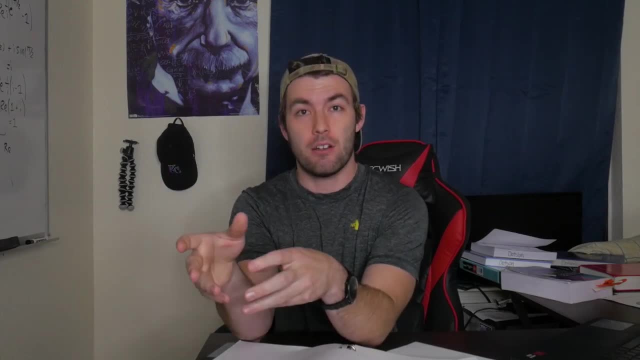 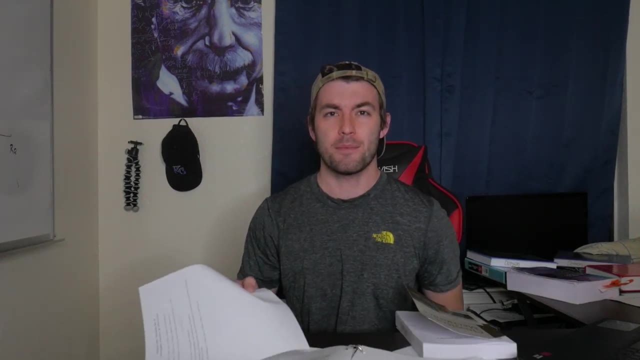 Lagrangian formalism, because the momentum being conserved doesn't necessarily mean that the generalized velocity is, so it doesn't really reduce the problem as much. Sorry, that was a bit of a tangent, but the problems themselves for the homework are almost all straight out of the 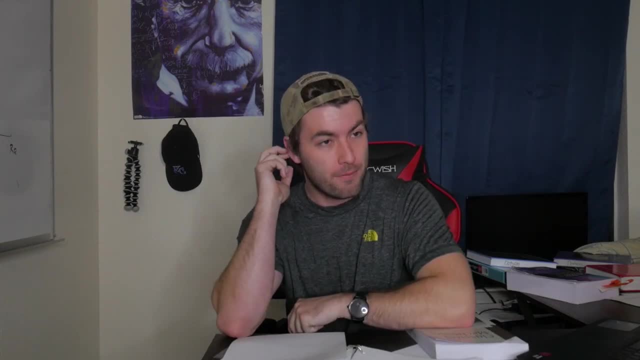 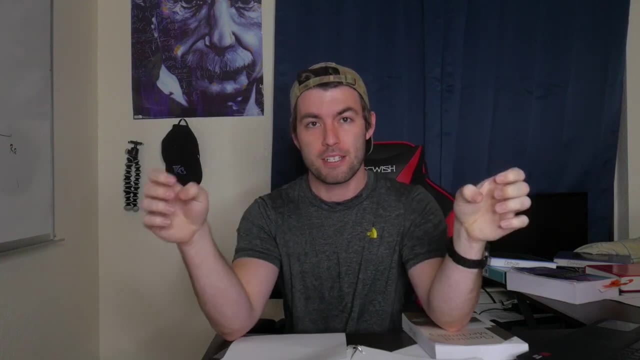 Goldstein book in chapter 8, and it's kind of what you would expect. It's a lot of find the Hamiltonian solve Hamilton's equations for this kind of system, For example for the central force problem or for two springs being connected.